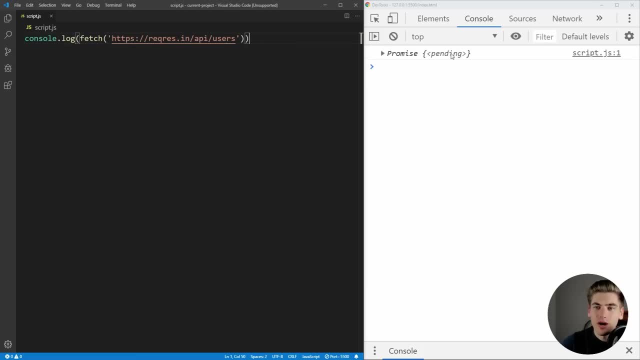 of Fetch And if we save that, you see that we're getting a promise on the side here. So we know that Fetch is promise-based, which means that we can use async await or we can use then and catch with it. And if you're not familiar with promises or async await, I have links in the description. 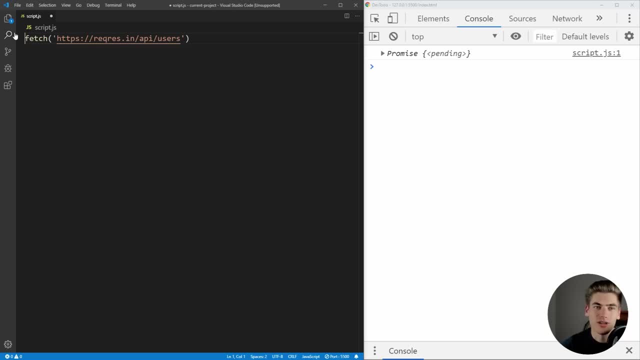 and in the cards that you can check out those videos that I've made on both of those topics. So, to get started, what we need to do is we need to say then, and Fetch is going to return to us a response, So we have a response object and we're just going to log out that response object to see. 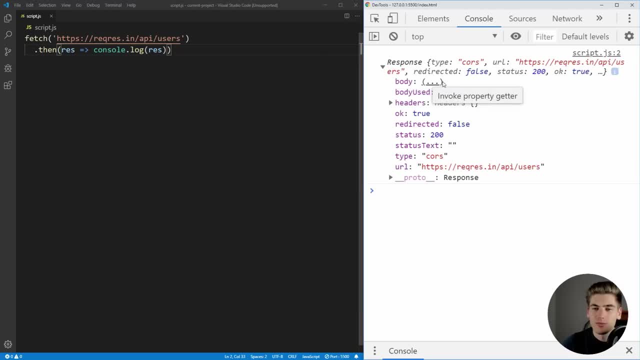 exactly what this looks like And if we save that, you see we get a response that says that the status was 200, says status text is empty. OK is true, so we know that this was successful and it has a body which is going to be all of our data, But this body of data is actually not. 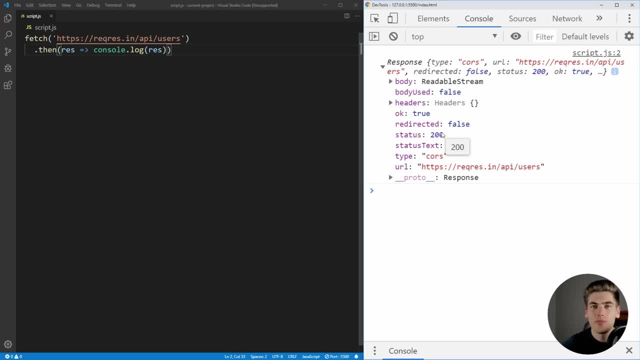 accessible directly from the response object. We need to call a method on it to convert this response to JSON, since we're actually using JSON data. So what we need to do is say resjson and this is going to return another promise. So then we need to use then 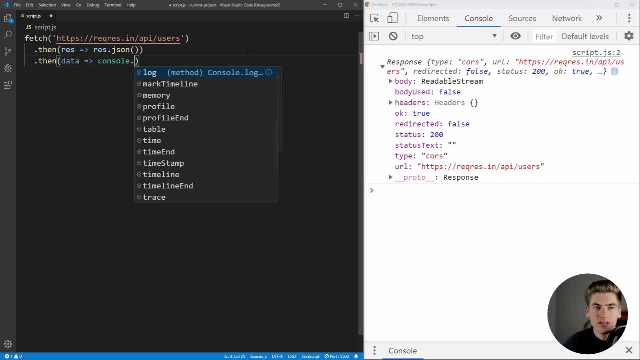 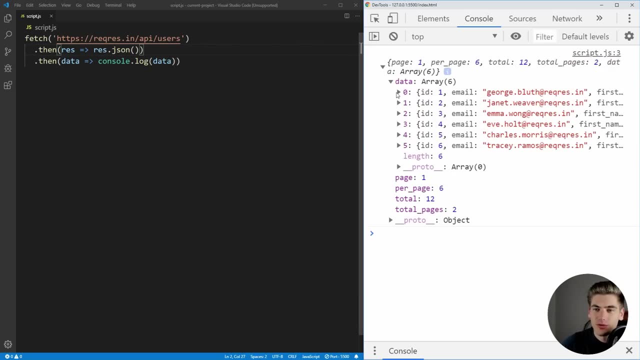 again and this is going to be our actual data And we can say consolelog of that data. So, as you can see, we have all of the different data on the right-hand side here. It has page numbers as well as all of the different users that we're getting from the API And that's working. 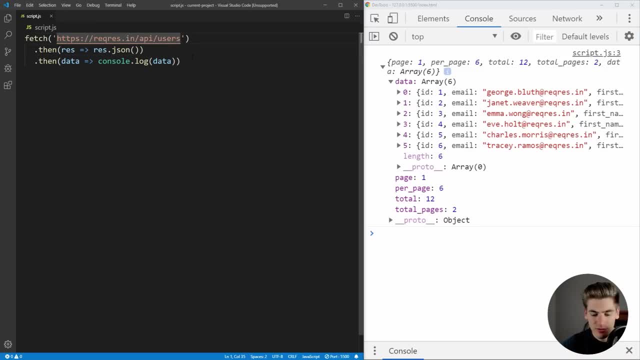 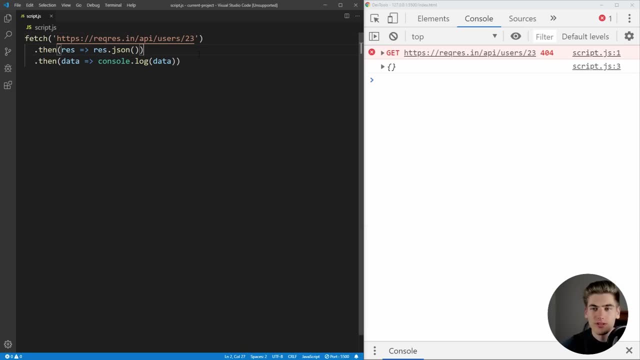 great, Everything's looking good. But what happens if we want to get a single user And, for example, we're going to get user 23, which does not exist? So we're going to get a 404 status back And when we save this, you're going to see that our get request actually happened. 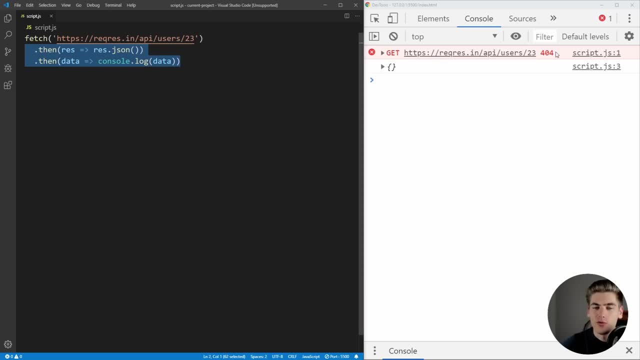 but we still ran our successful then code even though we had a 404 being returned. You would think that, since a 404 is an error, that it would end up in a catch statement like this, where we have an error, And then we would just want to log some text that says error. 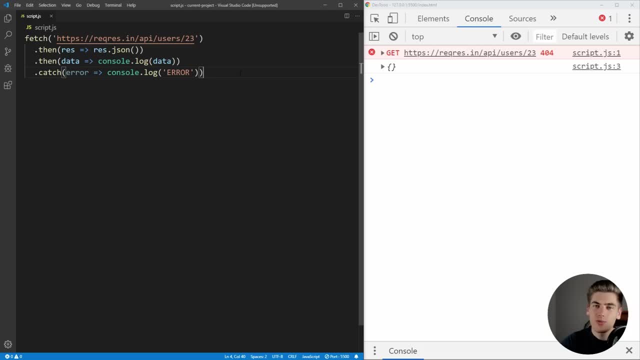 you can see we're not getting any error text, And that's because the way Fetch works, even though we're getting a 404 response, which is a failure of a response, always succeeds no matter what, unless there's some form of network error where 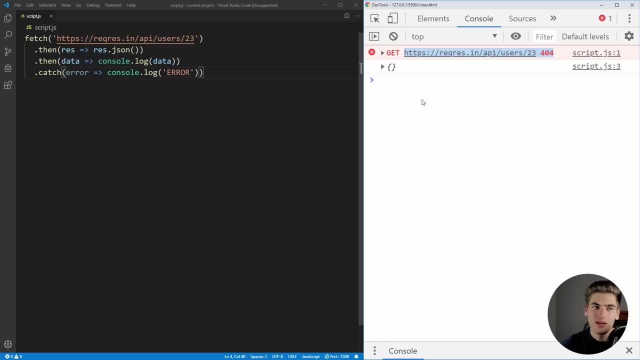 the actual browser has a hard time connecting to the internet. the only time you're going to get a failure is if you have the failure with fetch itself and not with the API you're calling. so what you need to do is inside of your response. you want to check to make sure the response is okay. so inside of here. 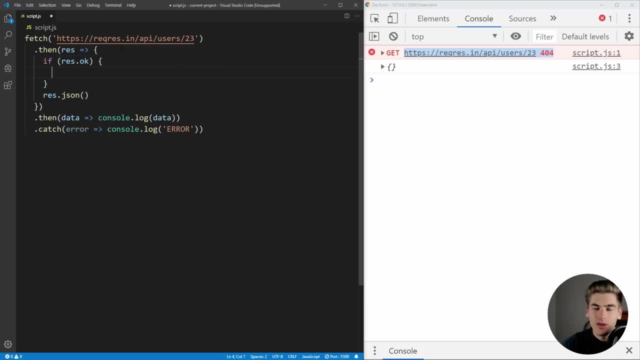 what we can do is we can say: if rez dot, okay, then we know we had a successful response. we're just gonna, for example, console out log success. else, if it's not successful, we're just gonna say something else. we're just gonna say: not successful, there we go. now. if we say that, you can see, we get not successful. 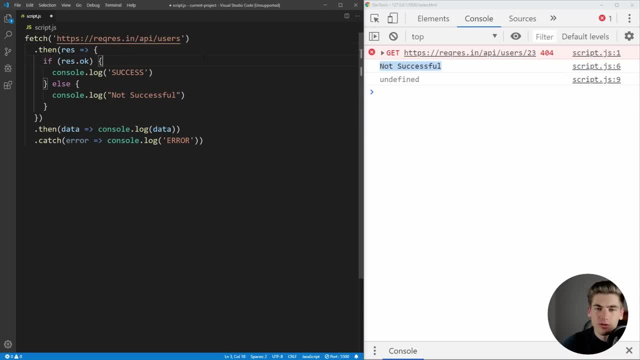 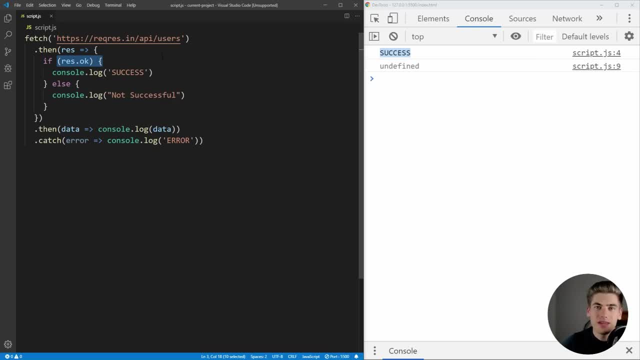 299. now, that's good and all, but with fetch, many times you want to do more than just get data from the server. you actually want to post data to a server, update data, delete data, and in order to do that, you're going to need to use the. 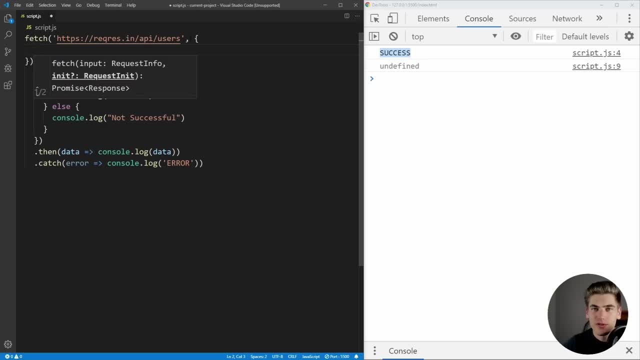 options section of the fetch method and the first thing we need to do is pass in a method. this can be either get post, put delete. it's just one of the HTTP methods. so in our case, we're gonna use post. we're gonna create a new user at. 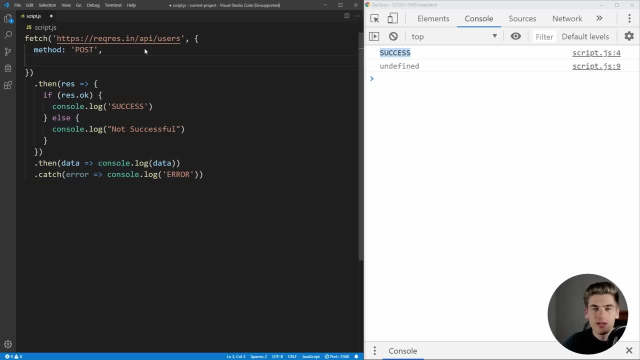 this API by just doing a post request and then what we need to do is we need to actually pass the data for that user and that's going to go inside of the body and we're gonna pass that as JSON. so let's just come in here and give the user a name and we can just say user one. 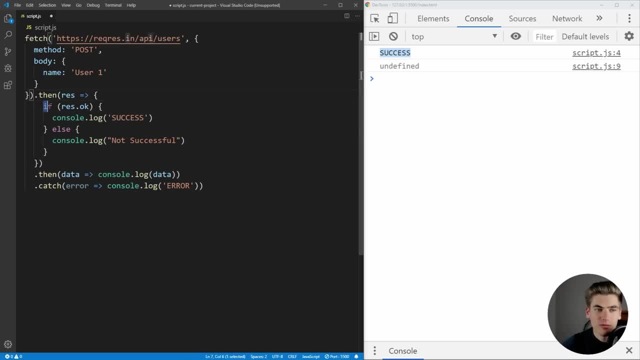 is the name and we can tidy up this code here. we can return just rez JSON. make sure we return that and there we go. now. if we save this, you're gonna immediately notice it's not going to work. we got our data back and it looks like it works, but 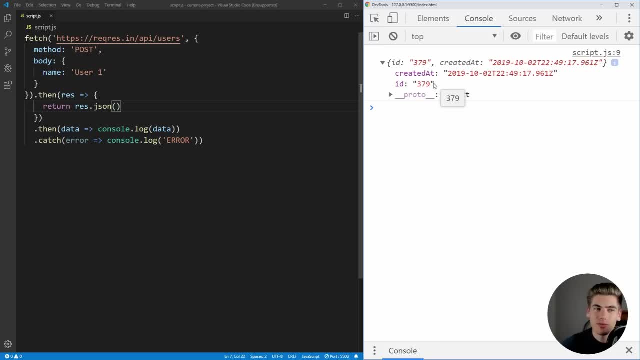 as you can see, there's no name for our user. it didn't actually save that as a name for our user properly, because this body didn't get sent up correctly. the way that fetch works is you actually need to send it JSON, so you need to do JSON dot.